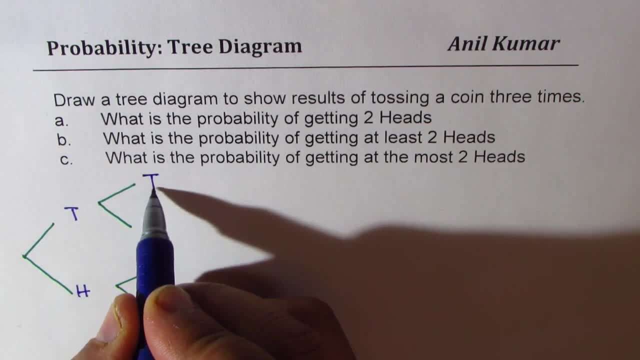 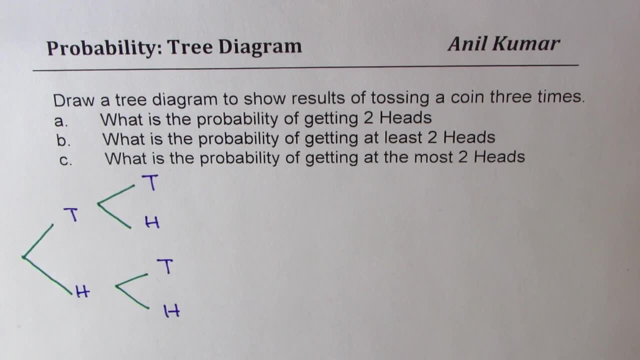 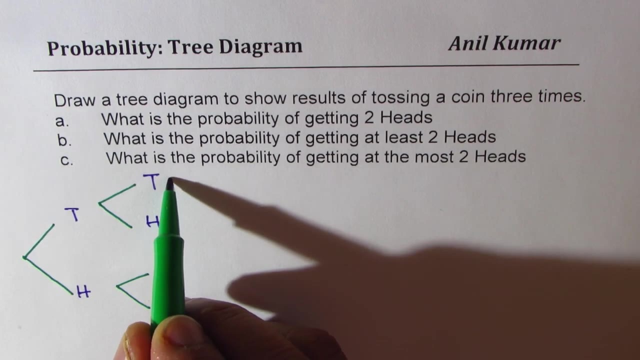 So we are also assuming that both are fair coins, That is to say that the probability of getting two heads is zero. The probability of getting a tail or a head is 50-50,. right Now, in the third toss, we may get a tail or a head. Let me write it down. 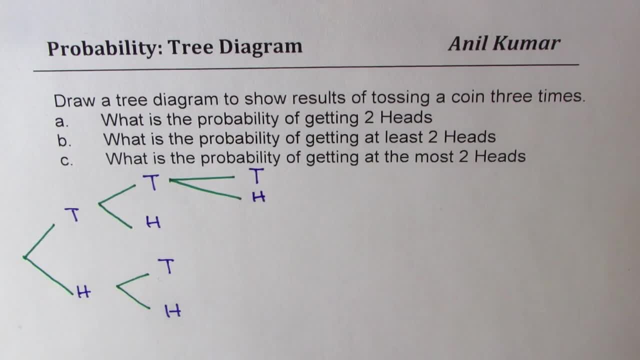 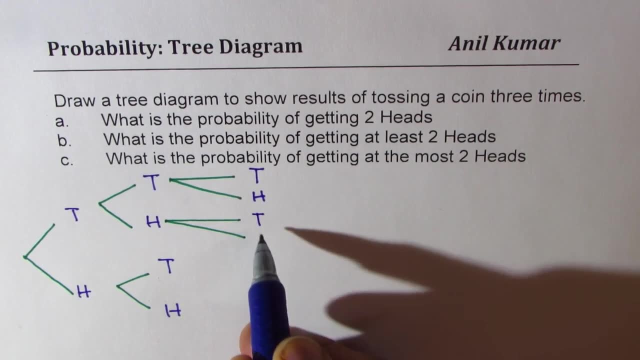 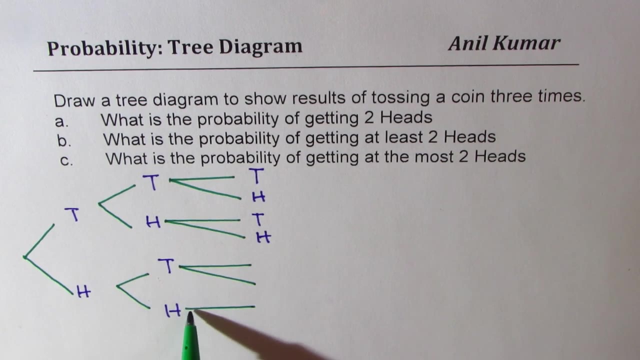 Here also, we may get a tail or a head. If we make two faces, we might get a tail or a head, since the probability is equally likely, right? So we could use both these terms: equally likely and 50-50.. 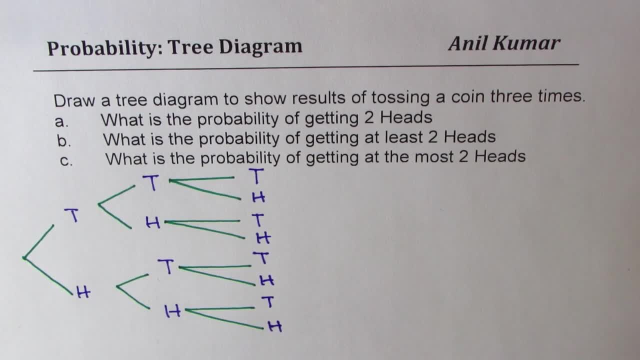 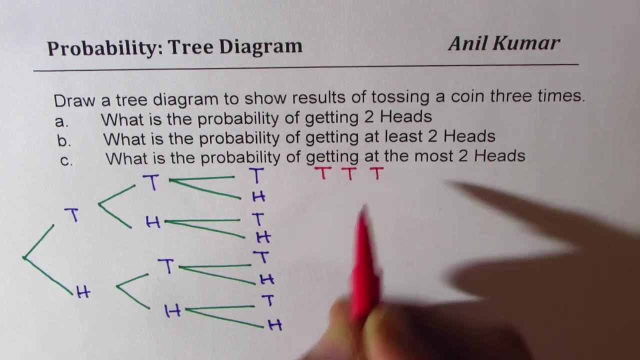 Okay, so that becomes the scenario. Now. what is the result of three tosses? So what you note here is that if we go with the first branch, we get all tails. so let me rewrite this as tails, tails and tails. now here we have combination. 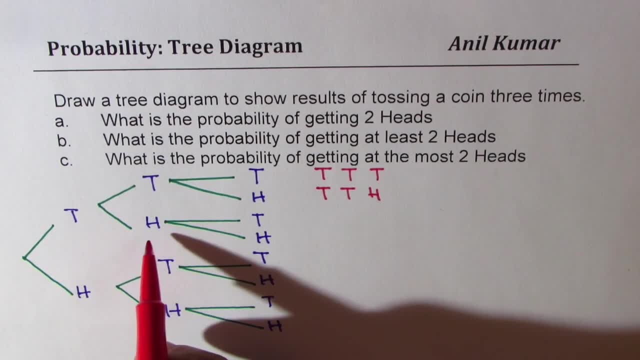 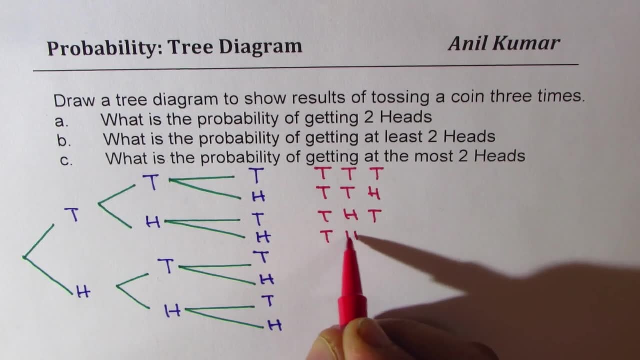 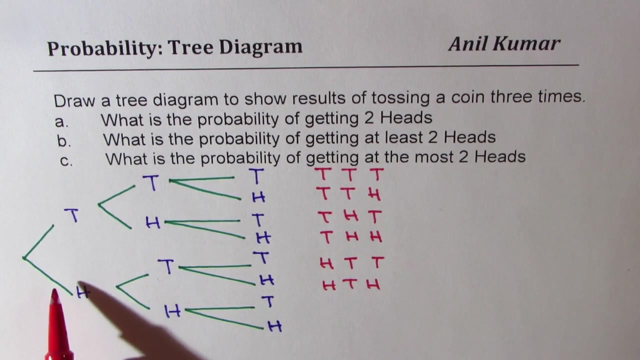 of tail, tail and head, then the next branch is tail, head. then we could get from tail head. we could get either tails or we could get head. now, if the first toss results into head, in that case the second could be tail and then with that we could have tail or we could have head. in the last case, if head is what we get, 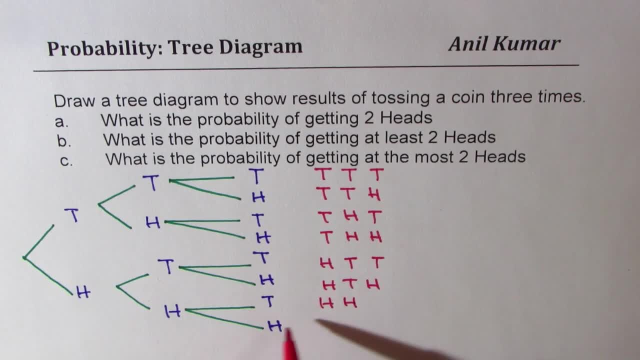 first. it could be followed by another head, after which we could get either a tail or a head. so these are all the possible outcomes, right? so so here we have all possible outcomes. so we say: number of possible outcomes is: how many is one, two, three, four, five, six, seven, eight? good, so that is the. 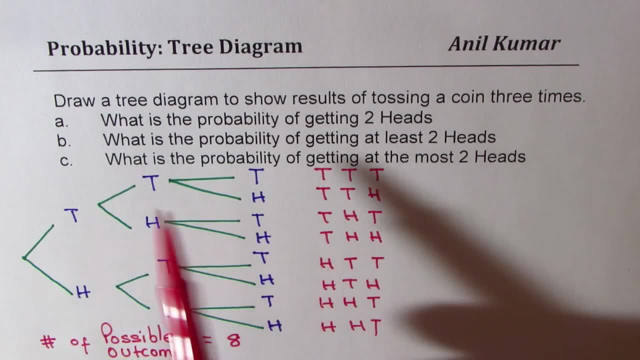 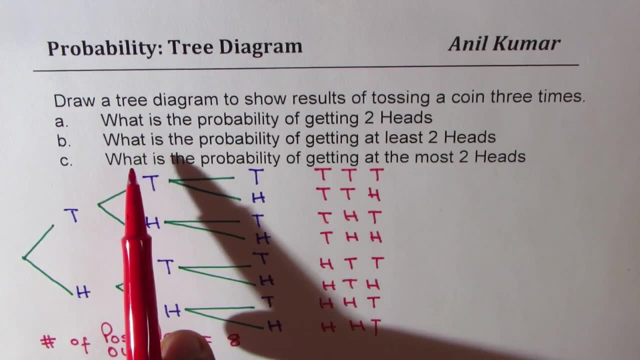 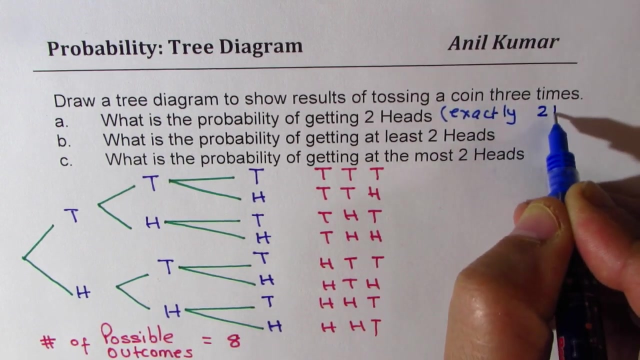 denominator for our probability. but now we'll take these cases one by one. what is the property of getting two heads? that means exactly two heads. what is the property of getting at least two heads? it means one or two heads. right, so that means the first question. it brings work. it means exactly two heads. let me write H. 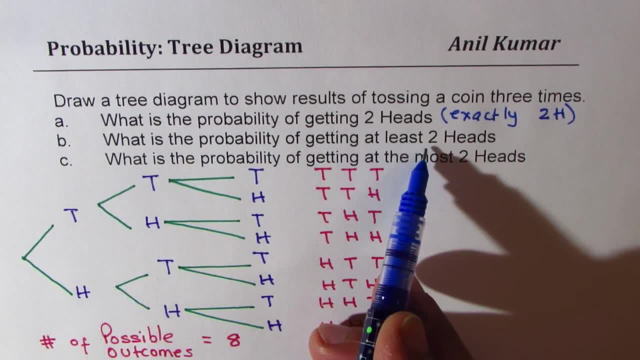 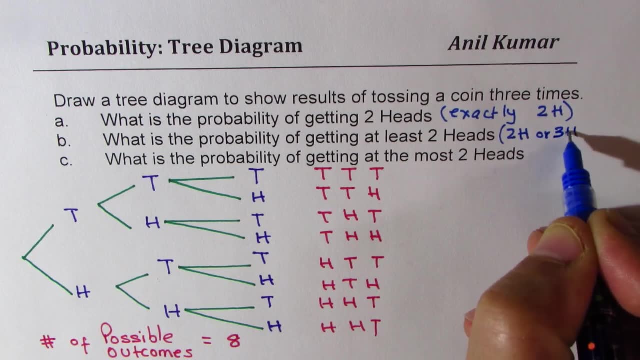 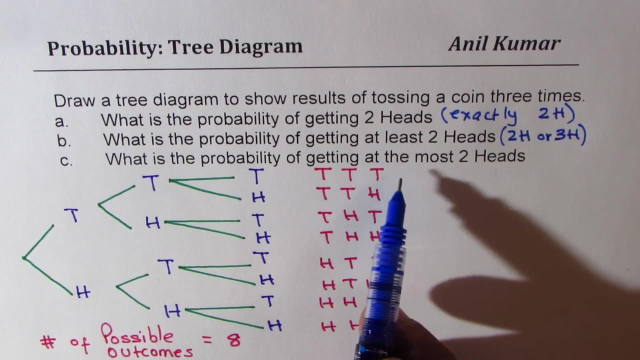 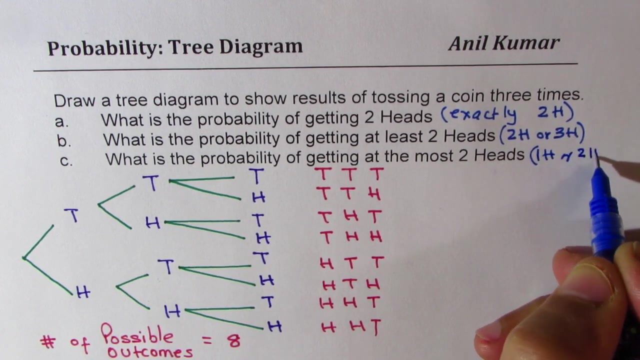 4 heads. what is the property of getting at least two heads means either we get two heads or we get three heads, right? so least at least two heads doesn't make sense to you. what is the probability of getting at the most two heads? that means We are looking for one head or two heads. 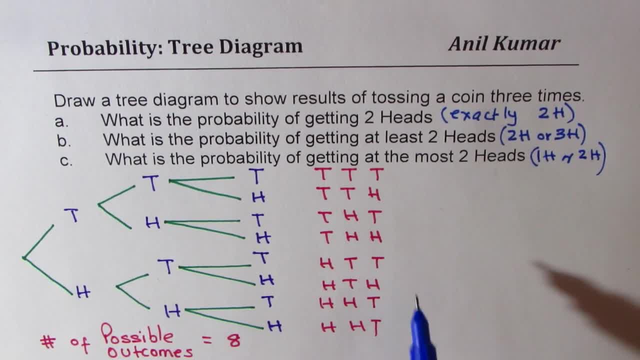 So these are three different types. Now to answer, it's a good idea to just make a table for heads. So let us say we want to find how many heads right? So heads could be either no head or we get one head. 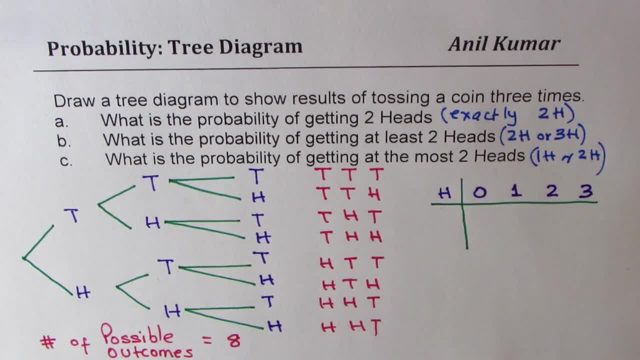 or we get two heads or we get three heads, correct? So let's count these numbers For no heads at all. I'm sorry, the last one was all heads. I wrote T here. This is all heads right. Head, head and head is all heads right. 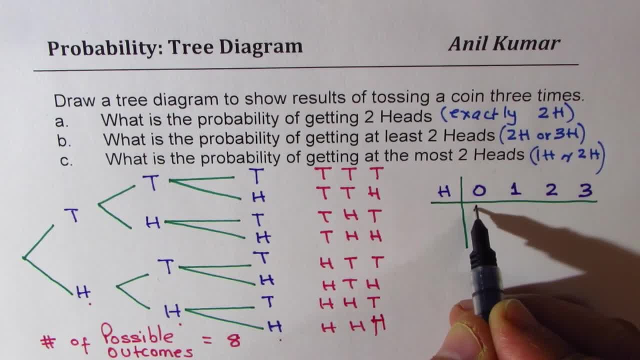 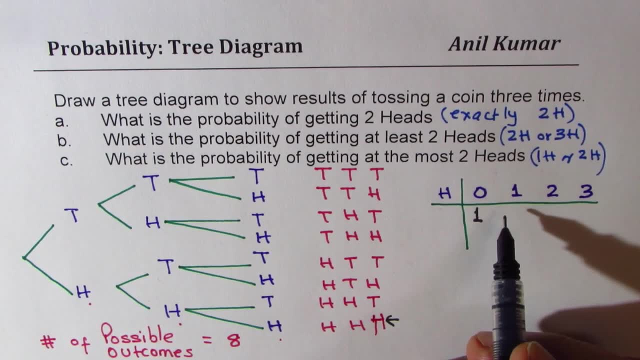 So for no heads. it is the last one. So we get one combination which is all heads, right. This one Now for just one head. how many combinations do we have? We have one, two and one three. 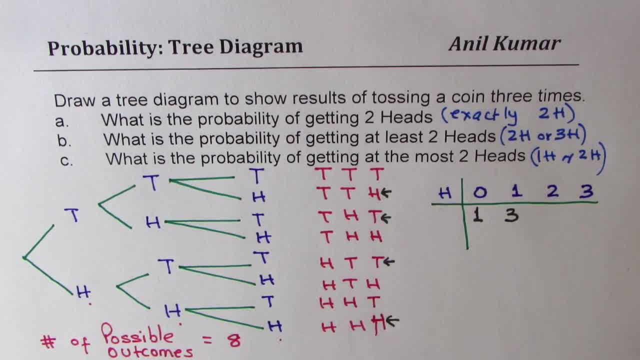 So there are three combinations with just one head. How about with two heads? So we have this with two heads, then we have this with two heads and again one more. So there are three with two heads, and I mean zero heads. was this one? 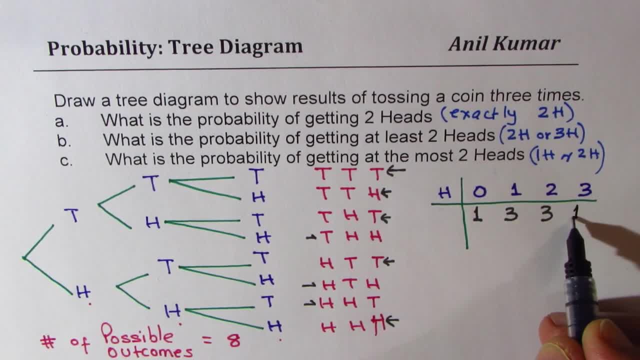 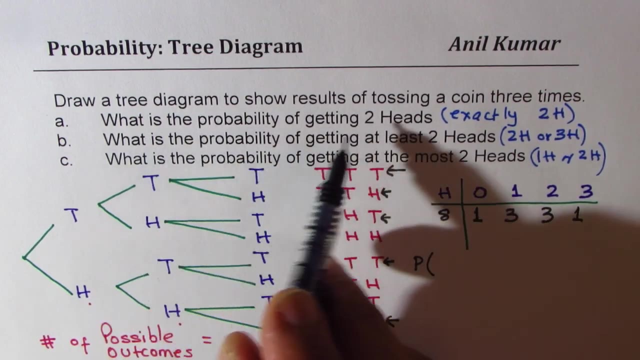 Sorry for that. Three with this one. okay, So in all we have eight combinations total outcomes: Is that clear? Now that becomes simple enough for us to answer the questions. So first one: here is probability of getting exactly two heads. 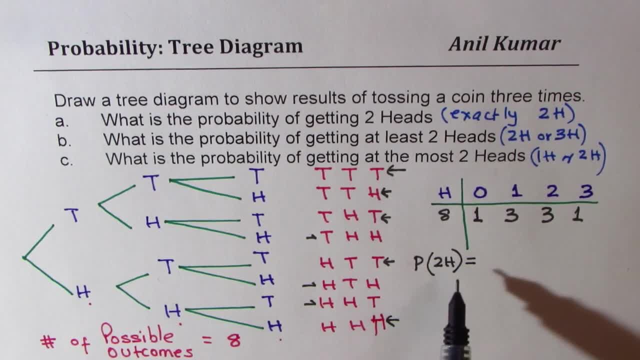 So let me write two heads. right is how much So two heads will get. there are only three ways. Okay, So favorable outcomes. So favorable outcomes is three and total possible are eight. So we get three out of eight. 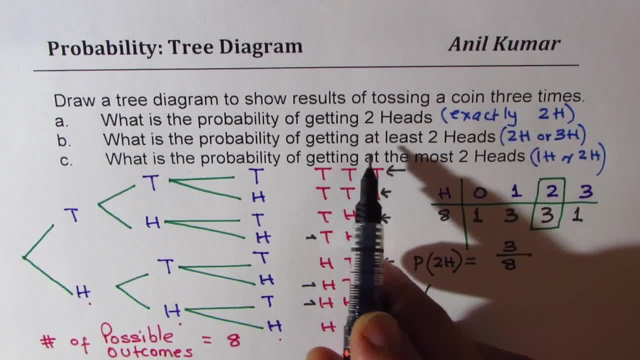 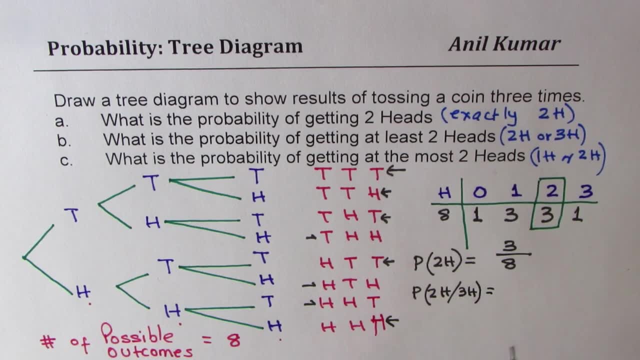 Now for part B. probability for getting at least two heads means either we get two heads or we get three heads, So two or three. So we have to combine these two cases. So three plus one is four, right? So we get four out of total of eight. 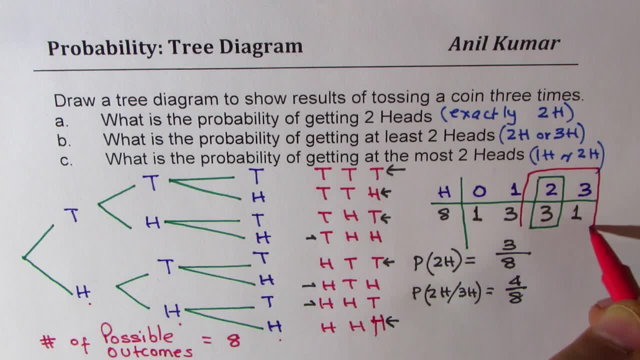 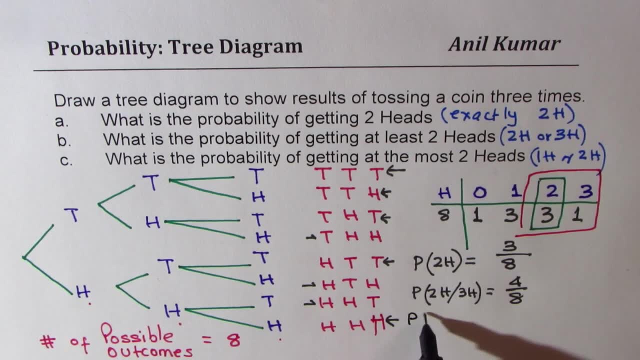 So for this we combine these two. Do you see that part Two or three- Now the last one is at the most two heads. That means we're looking for just one head or we are looking for two heads. So that is at the most two heads. 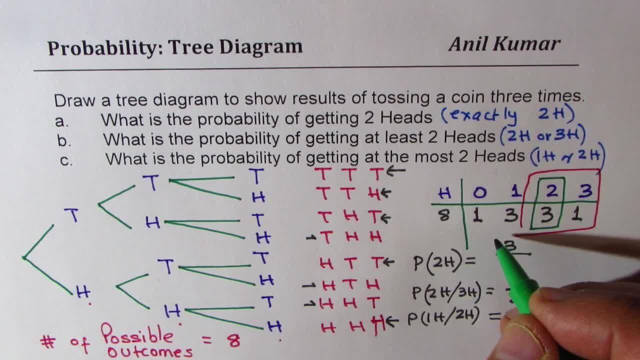 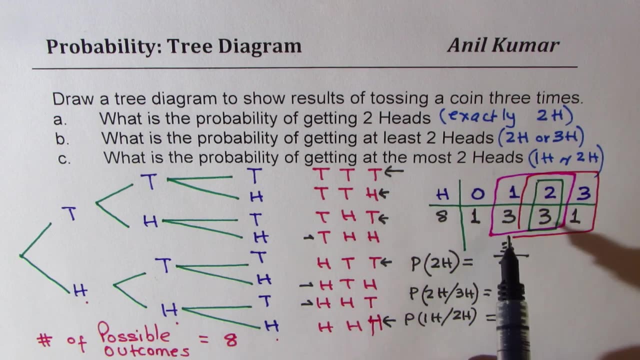 So now we are looking for one or two. So that means we are looking for the combination which is- let me use a different ink- One or two, which is this combination. So how many are there? Three and three, six. 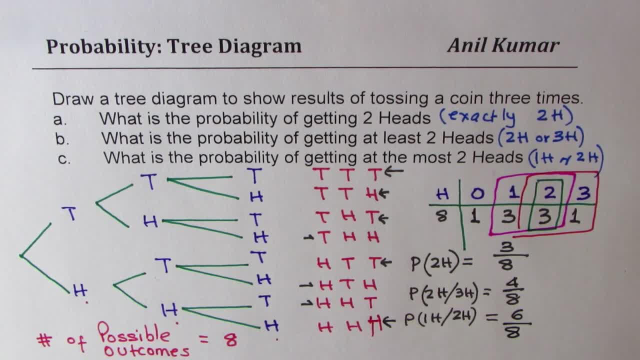 So this answer is six out of eight. Perfect, So purposely I'm writing this in this way, but it could be always reduced to lower value, So it is good idea. So four over eight should be written as half or 50%, and six over eight could be simplified.